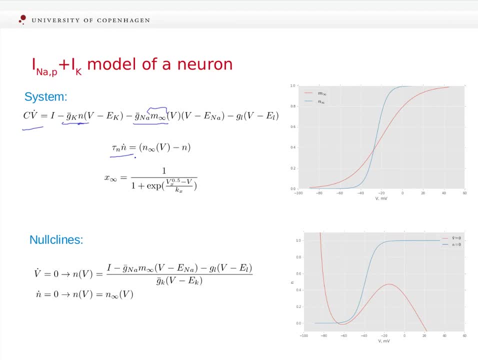 plane. So both potassium and sodium currents have their own voltage dependencies And they are depicted in this figure. So this is for the sodium current and this one is for the activation of the potassium current. And in this figure we also see the steady state activation variables for each membrane voltage. 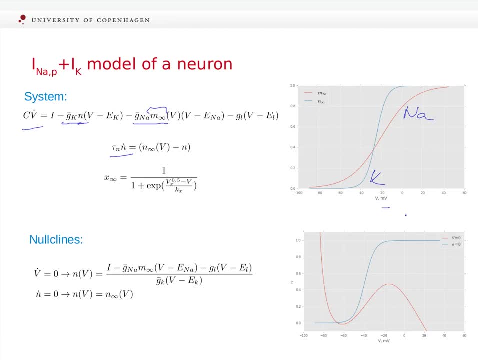 And the HD oficial side of each membrane is P treasure and we can see that when the neutrin is or não is twelve processed. so in our sum we can called thatekenutron. The non-cline for this model are easy to derive analytically and they are 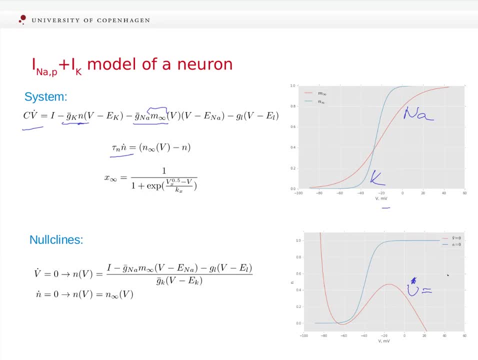 shown in the bottom graph here. So these are the non-clines. The red here is the nook line- novels idolized in this question- And of the membrane voltage, and the blue one is the node line of the activation gate of the potassium current. note that any change in the amplitude of the applied 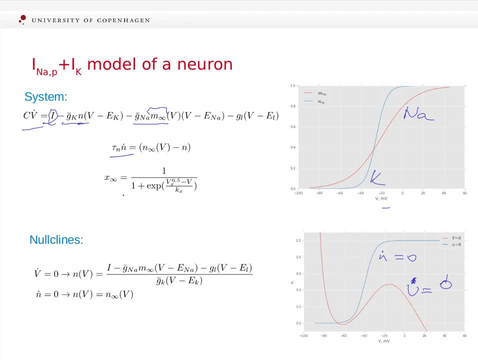 current here. so this is the current we stimulate our neuron well. so any change in it will just shift the V nook line upwards or downwards depending on the sign of the applied current. so the polarizing currents will shift the V nook line up and hyper polarizing currents will shift the nook line down. 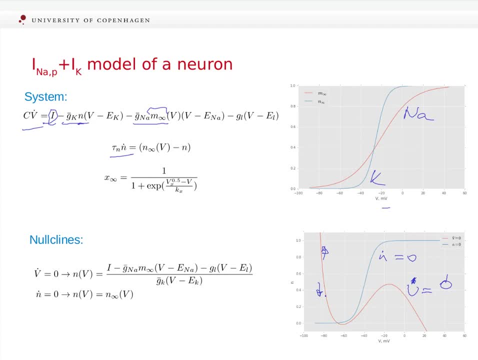 and well, this will will define the change in behavior hours of our dynamical system, and the actual shape of the nook lines will define what kind of bifurcations they will be occurring. intersections of the nook lines are, of course, fixed points or equilibrium- just one here, for example- and they can be either stable or 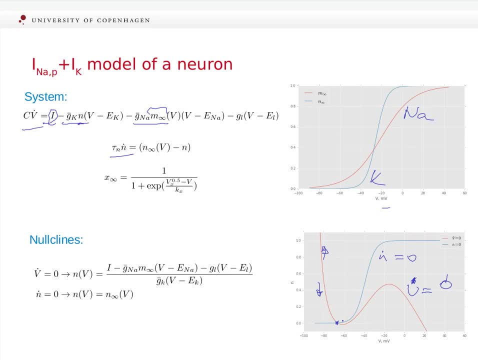 unstable, depending on the corresponding eigenvalues. just as a quick reminder, all phase projectories will cross the view, the v-noot lines vertically and will cross the n-noot lines horizontally, And of course, any point on the phase plane is the state of a dynamical system. 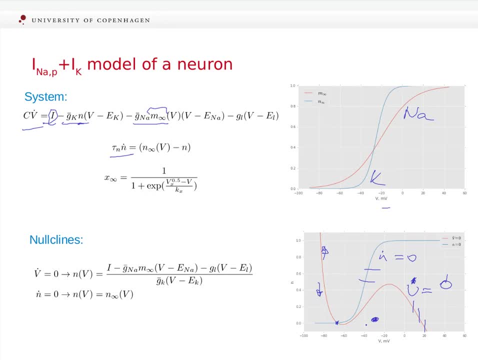 I should note that this model is practically equivalent to the well-known Morisly-Karr model of the giant barnacle muscle fiber, except that there is a calcium current in the Morisly-Karr model and sodium current in this model. This model is kind of simple and doesn't have a lot of equations, but it still captures. 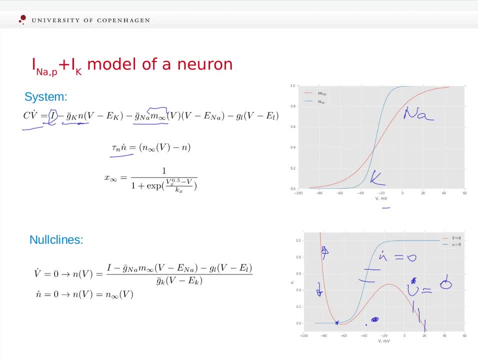 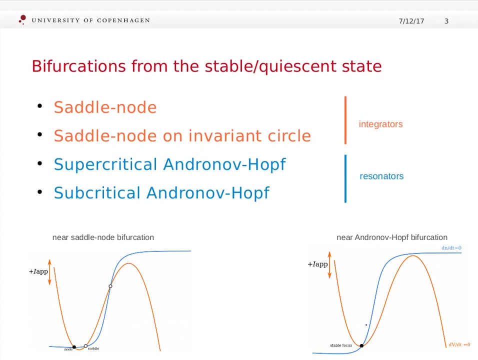 the main properties of neurons, main excitability properties of neurons, And we will discuss this right now. So a change in number or stability of an equilibrium point leads to a change in system dynamics and it's called bifurcation. Let's look in more detail how a model neuron can switch from a resting state to periodic. 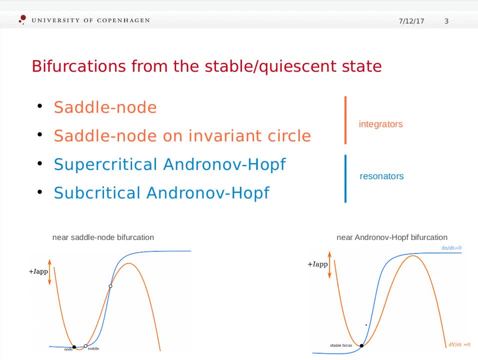 spiking. If we allow the change in only one parameter, for example the applied current, then the neuron can lose stability. So if we change the Datum value of the neuron, we can turn the neuron's stability via one of the four scenarios, depending on the values of other parameters. 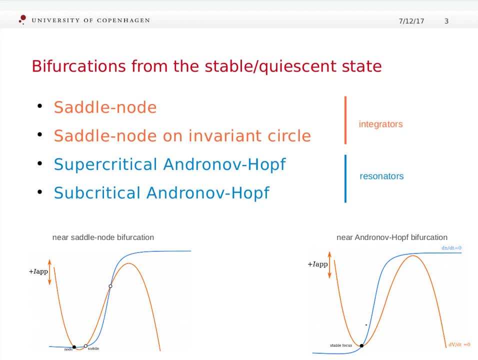 As we shift the null-client up, the two equilibrium points, the stable node and the acetyl, can merge together and annihilate, leading to a creation or a jumped-tour limit cycle. So these are the two bifurcations. 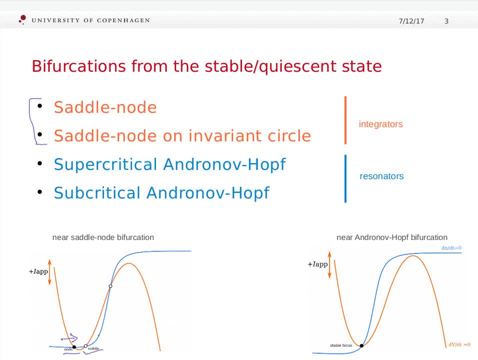 and a saddle move towards each other as we shift the wheel-mute line up and annihilate, and therefore the system can't dwell here anymore. it will either jump to an existing limit cycle or the limit cycle will be created. presently, these two bifurcations are called saddle node bifurcations. 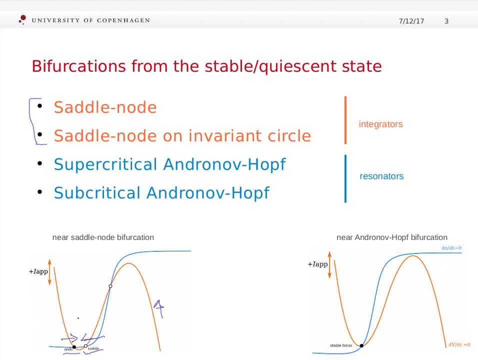 and neurons near these bifurcations display certain neurocomputational properties which allow to call such neurons integrators. and when i say neurons near these bifurcations, what i actually mean is that the actual physical properties of real neuron can be described by a dynamical system where the parameters organized in such a way that the data 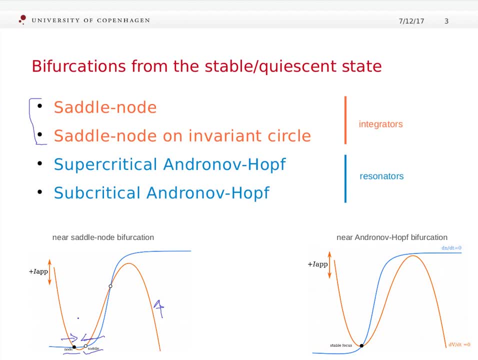 system is near the saddle node bifurcation. On the other hand, for example, when the potassium current activates at more hyperpolarized membrane voltage, so it's more sensitive potassium current, there is a single equilibrium point, namely a stable focus, so all trajectories will rotate around. 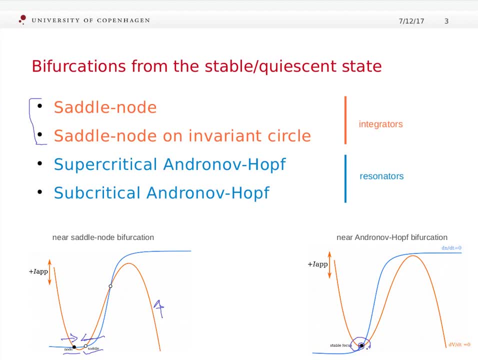 it and finally fall on it. so it's a stable focus. then it loses stability and becomes as unstable as we shift the V-node line up or inject a dipolarizing current in a neuron, Depending on the condition, if there is already an stable, 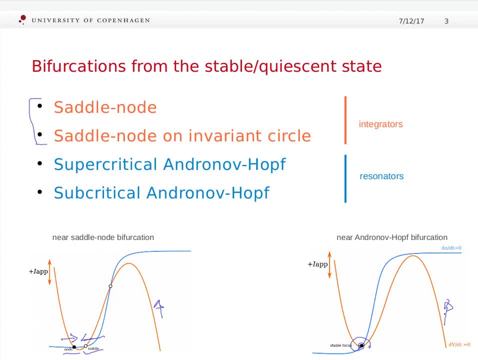 limit cycle attractor at this moment or it is born simultaneously. the bifurcation is either subcritical or supercritical Antonov-Hopf bifurcation respectively. Because the neurons near such a bifurcation have dumped subthreshold oscillations, these neurons can be called resonators. It is important to note that. 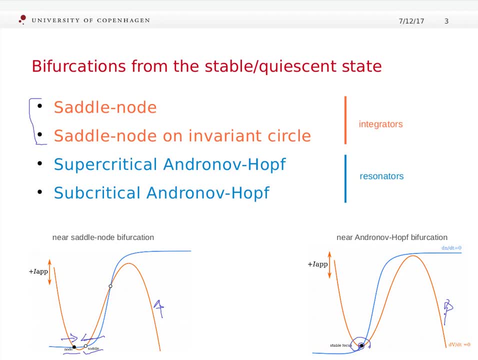 although we use the simplified model to demonstrate the bifurcations, any dynamical system can switch from resting to spiking state or oscillations via one of the four main bifurcations described here, And this is in the case that the bifurcation is co-dimension 1, that is, it is brought 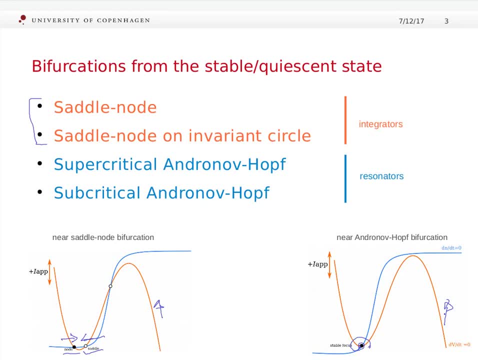 about by changing a single parameter, while arguably such a situation, when a change is only required in a single parameter, is more likely to happen in nature, in real neurons, than bifurcations requiring simultaneous change of two or more parameters in a coordinated manner. 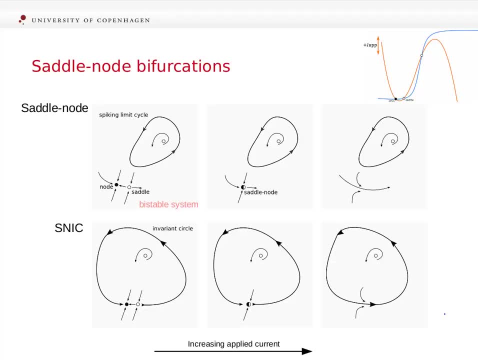 Terrible hipo is that an feel-alike procedures in a single Ray 배 can be desired. An echoing faculty of service can also make the patients change in their own Brazil ethics. But there is one exception: vacancies. That's the sixth option. In both cases the nodes move towards each other and coalesce, resulting hour: subtle node fixed point, which is a saddle on one side and is an unstable and stable car-a- einen dire des von Here. The antenna focused on pole, SEO And a couple of other cos. 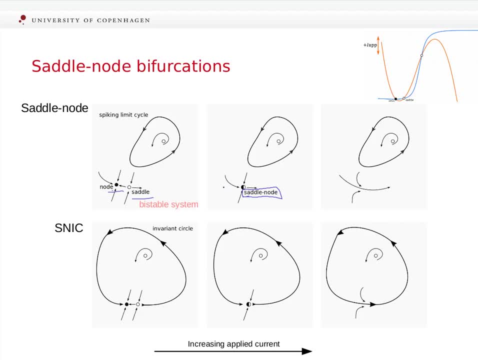 Let's see if this is thinkitet, while we're staying in, of the single parameter惕 table and a, so to speak, node on the other side, And that's why it's called a saddle node or fold verification. So there are two scenarios. The one scenario, 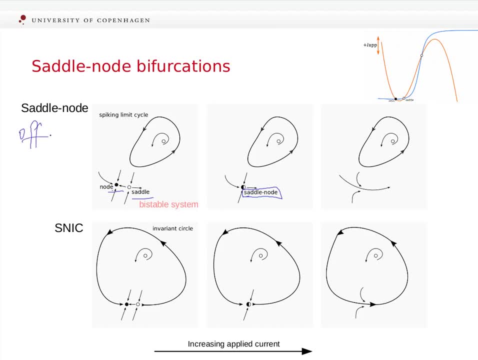 which is called a saddle node of invariant circle, that's, that's a C here I'll make it right, that's of invariant circle. and this is a bistable system, meaning that although a neuron can be in a resting state- quiet, not spiking, but 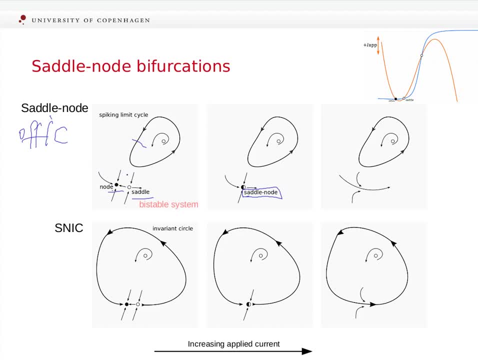 this stable state has a limited attraction, a basin of attraction. So it's a stable state and the neuron can be in a resting state or a quiet state. So it's a stable state and the neuron can be in a resting state or a quiet state. 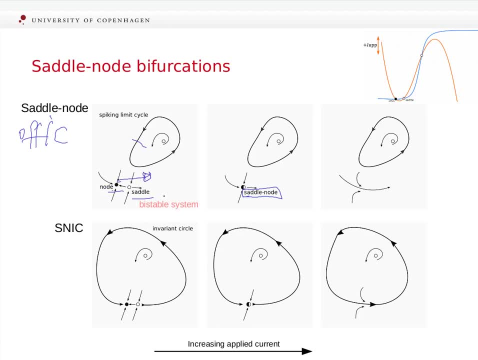 So if we, if we suddenly stimulate a neuron with a short pulse and move its state horizontally along the V axis, it will then find another stable attraction, which is here a limit cycle. So another stable attractor is a limit cycle, which is here a limit cycle, and it will be spiking. So depending on where we 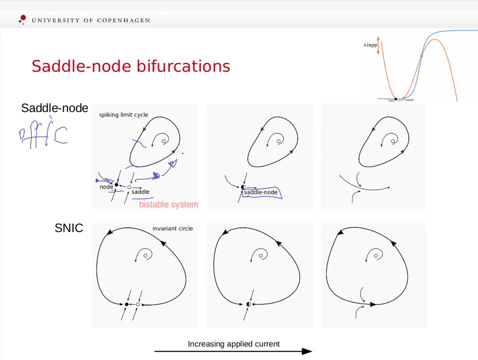 start. either we start near the node or either we start in the attraction basis of the limit cycle. we will get either sustained spiking or resting for the same combination of parameters, And this coexistence of two different kinds of behavior is important for, for example, 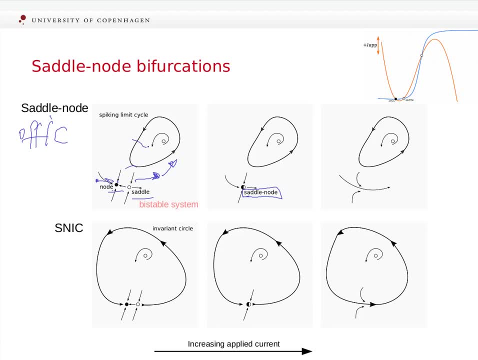 bursting of a neuron that is spiking in short or long batches of spikes interleaved with quiescent periods. In the other kind of the saddle node bifurcation, the limit cycle attractor is born simultaneously with the vanishing of the saddle node equilibrium. 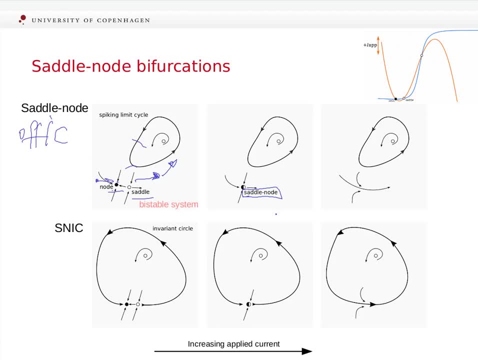 So this is saddle node on invariant circle. What happens here is, at the moment of bifurcation. we have this saddle node, equilibrium point, and any trajectory that will start from this side of this point will end up on the other side of the same point. 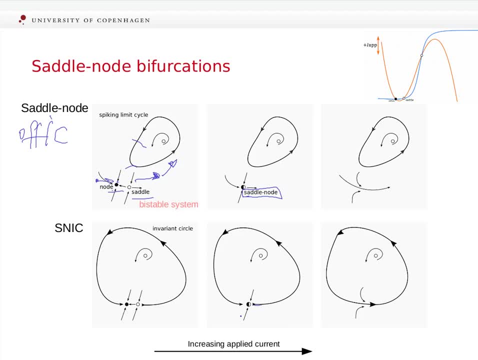 And this kind of trajectory is called an invariant circle. This can also be regarded as spiking at infinitely small frequency, because we start here, produce a spike and end up in here. So in time it would look something like this: We produce a spike. 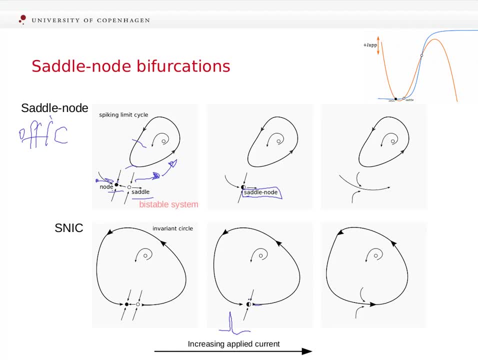 We end up in here. We produce a spike And then a frozen at the stable part of the saddle node. Finally, just after the bifurcation, we have a limit cycle. but near this area our system goes near both of the nullclines, as we shall see in the next slide. 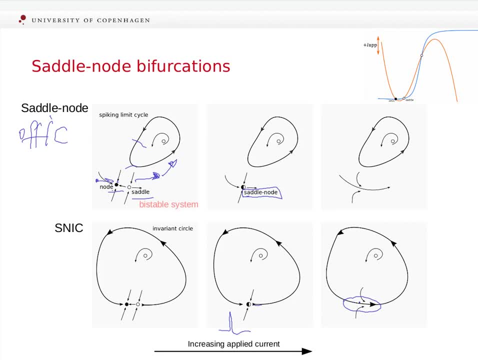 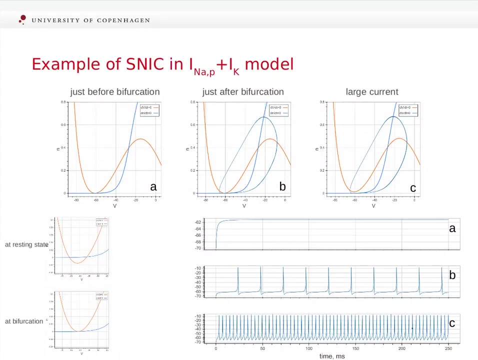 And because it is close to both nullclines, the behavior is very slow here. so this kind of slow valley, And this is manifested in very low frequency spiking, so the interspike intervals are very long here. This is illustrated in the following slide here: 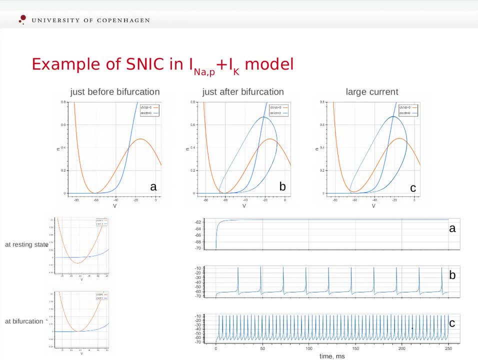 This is an example of a saddle node on an invariant circle bifurcation for our model, And this is the result. And this is the result, And this is the result. If we look at the zoomed up parts here, what we see- that at resting state we have a saddle. 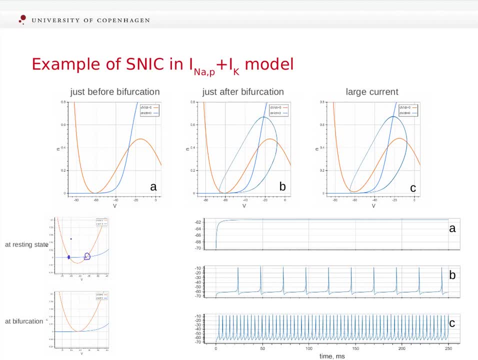 we have a node, we have a saddle and all trajectories, whenever we start, will be pulled towards the node And just after the bifurcation. we don't have any equilibrium points here and all trajectories will just pass this small valley here. 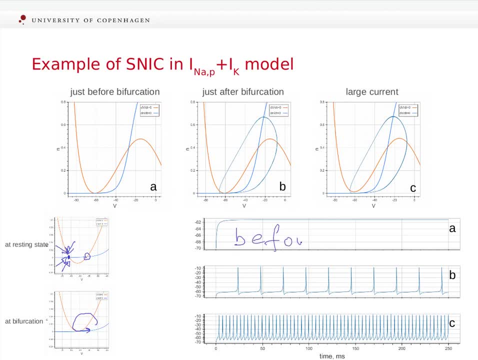 So this is just before bifurcation, this is just after or at, And this is way after bifurcation. so we increased a lot of the polarizing current in here and the separation between the two nulc lines is more. So this is the v-nulc line and this would be the n-nulc line here. 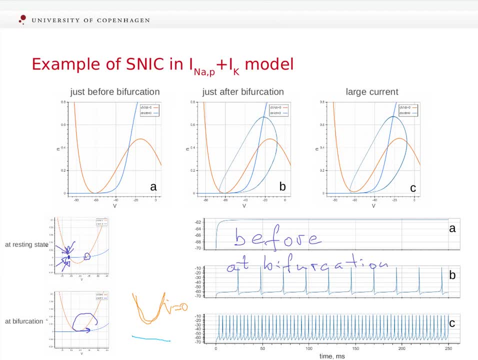 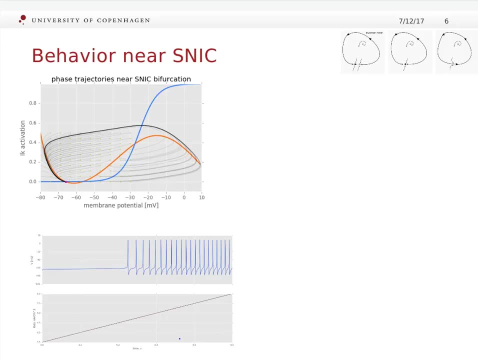 And a trajectory will pass here freely, as we will see in the next slide. So here I depicted behavior near the saddle node on invariant circle bifurcation. This is just before the bifurcation and this graph here shows that if we start at different parts of the face plane, 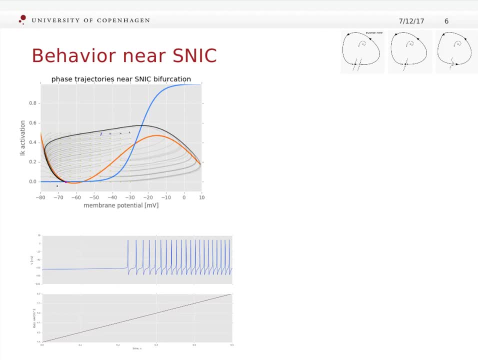 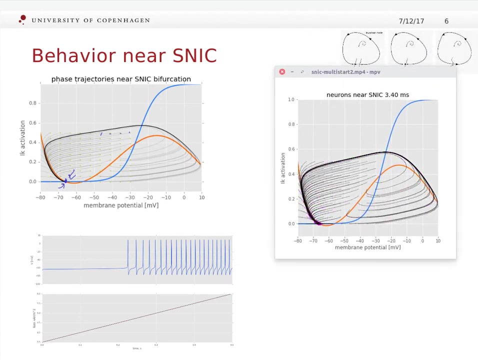 it doesn't matter where we start from. we will converge to the stable node. So this would be our stable node And, if everything goes right, I can show it in a video. So this is the video. Our purple points are the state of the system and the fading black lines are the trajectories. 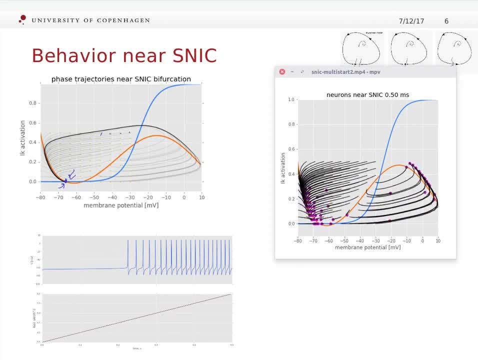 So it doesn't matter where we start from. we end up in the stable resting state. Now what happens if we gradually increase the applied current? This will move our v-nuclein up, of course, and we will observe the bifurcation. 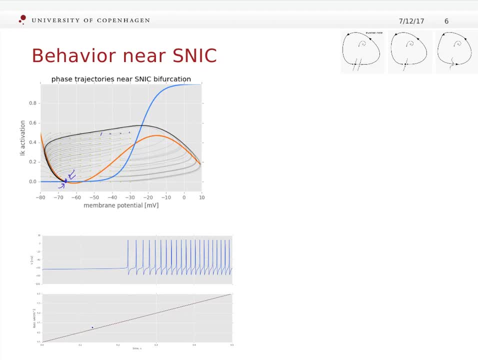 And this is shown in the graph here. So here we increase the applied current. This is our applied current. At first we are at the resting state, but then this resting state, the stable node, loses stability. No, it doesn't lose stability, of course. it just merges with the saddle. 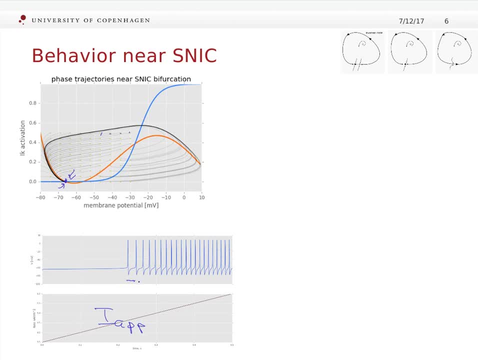 At first we have quite large interspiking intervals, which would be slow spiking or spiking at a low spiking rate. But then as we increase the applied current, the spiking rate becomes high and higher, or interspiking intervals become smaller and smaller. 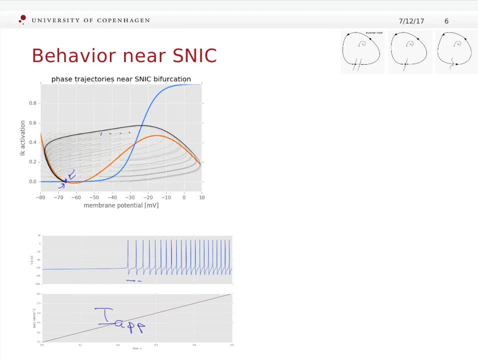 And I'll try to show it in a video too. So this is how it goes. Let's start from the beginning. So at first the system dwells in a resting state, but we are actually pulling the v-nuclein up And you can see that the system slips. 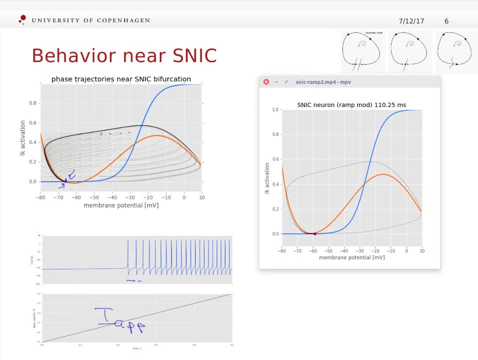 through the slow valley between the two nuclines And you can actually see how it slows down in this slow valley But then it produces the rest of the spike quite fast. But as the separation between the nuclines gets larger and larger, you will see that. 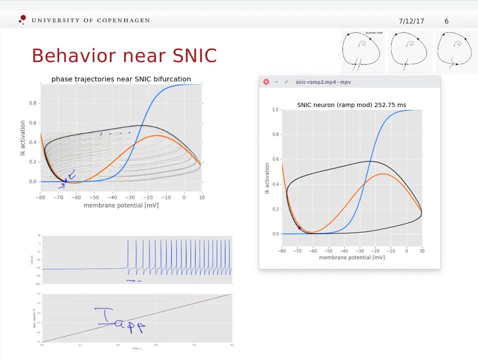 it takes less and less time for the system to go through this valley. All right, we see that the spiking rate increases. How lovely. Now let's look at the saddle node bifurcation of invariant circle, which we'll do in the next slide. 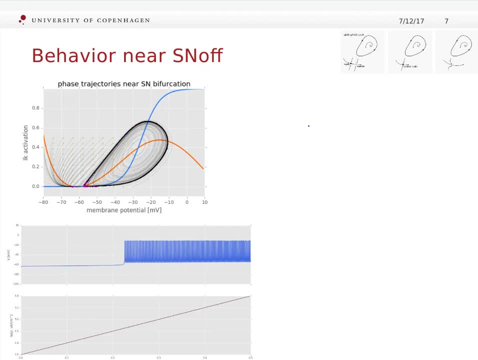 In here. these are the equivalent graphs. So we start our system at different starting points shown here and we either end up in the resting state or we end up in a spiking state. So these trajectories will move to the spiking state and these trajectories will stay on spiking. 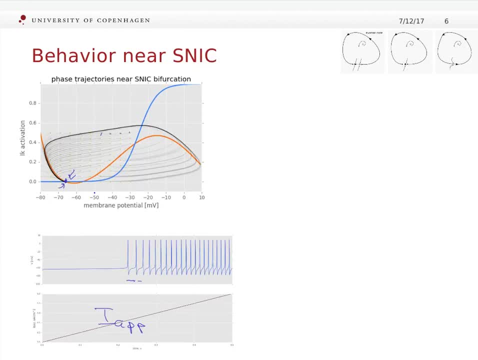 And one thing I forgot to mention in the previous slide: that the threshold of the excitability threshold for this kind of a neuron is actually the separatrice of the stable or of the saddle. And let me show it here: Yeah, so So this is it approximately. 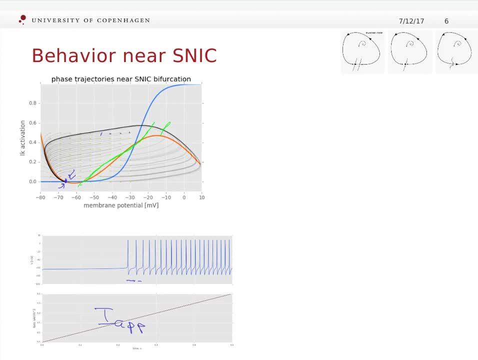 So the threshold for a neuron is not a fixed value of membrane potential, it's actually a line or a more dimensional manifold. If we start left to this line, we will have a subthreshold response. So we have something like this: 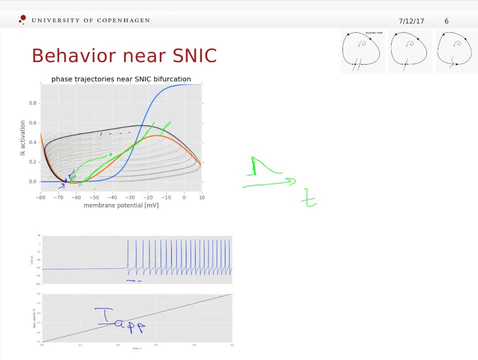 So if we start from here or very fast move the system from this state to this state, what we will observe is a typical excitability. we'll have an action potential or a large excursion over the phase plane like this, and we will end up. 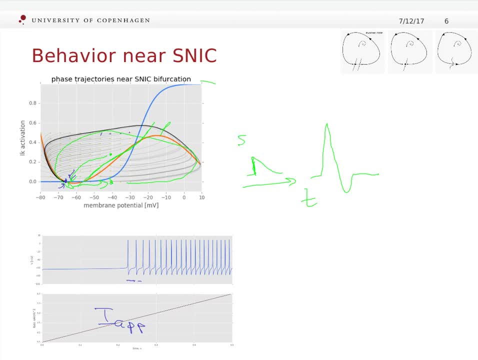 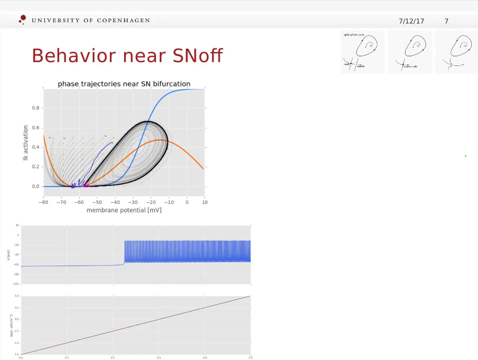 in the resting state. So this would be subthreshold and that would be suprathreshold. Right, so back to the saddle node of the invariant circle. And it is a bistable system. Let me make start of wieder and start it over. 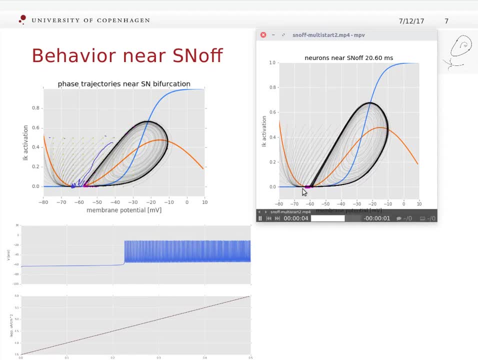 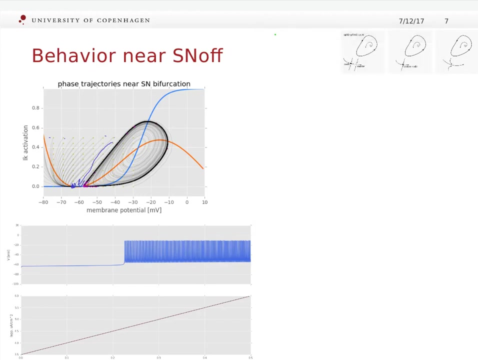 So we start from different parts and you see, some of the points converge to the stable equilibrium, a resting state, and some trajectories stay on spiking Right. so how the neuron near saddle node of invariant circle bifurcation switches from resting to spiking. 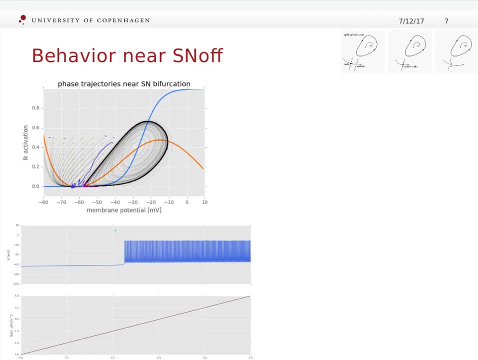 Right. so how the neuron near saddle node of invariant circle bifurcation switches from resting to spiking If we gradually increase the applied current, In contrast to the previous case where we observed a gradual increase in spiking rate, we don't see it here. What we see is an abrupt 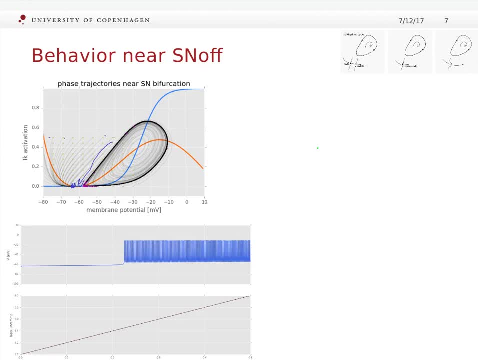 switch from resting to spiking at fixed or almost fixed and high frequency. So let's see it in the video, Right? so this is the right video. At first we are at the resting state, but we gradually push our V0-clan up and here we go, spiking at a high frequency. 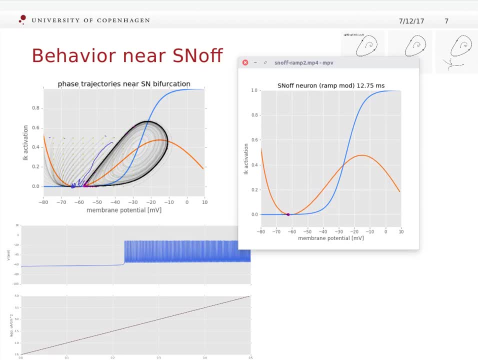 And please note it will be important later that as we spike we actually spend quite a substantial amount of time in this corner. so it's kind of a slow corner because it also is near both nude lines. Now let's consider the case of the Andronov-Hopf bifurcations. 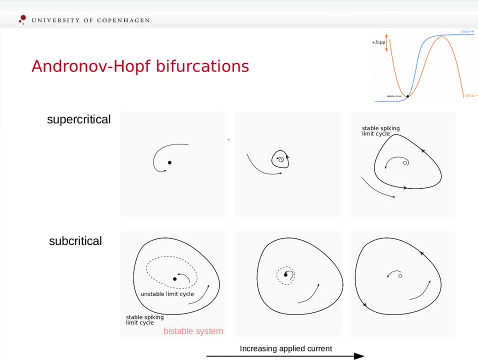 So again, there are two kinds of Andronov-Hopf bifurcations. One is supercritical and the other one is subcritical. In a supercritical Andronov-Hopf bifurcation we start with a stable focus. 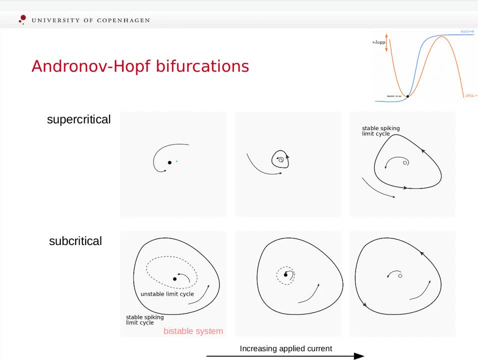 and all trajectories will revolve around it, with a smaller and smaller amplitude, but then the stable focus loses stability, which means that the real value, the value of the eigenvalues, changes sign and from being stable it becomes unstable, and we see that there is a small limit cycle around here. 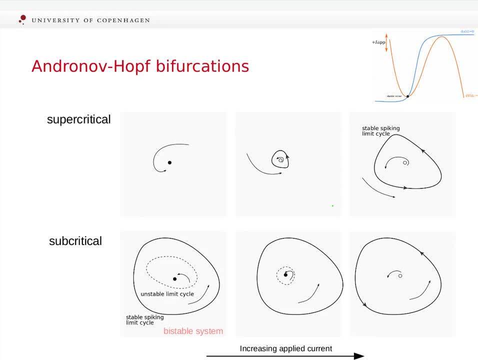 around this unstable focus. now, As we increase the applied current, this limit cycle becomes larger and larger, which means that we have larger amplitude spikes. So finally we have full-fledged action potentials, but before that we have kind of subthreshold or partial amplitude spikes. 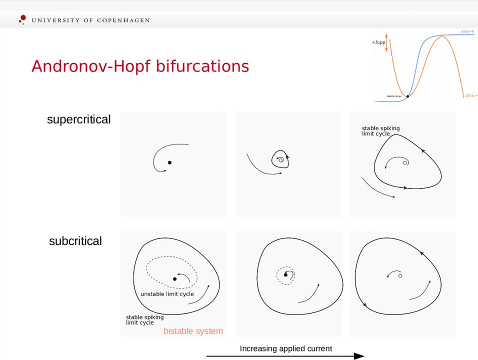 Now in the subcritical Andronov-Hopf bifurcation. our stable focus in here has a limited area of attraction and this area of attraction of the stable focus is limited by an unstable limit cycle, so all trajectories run away from it, rotating. 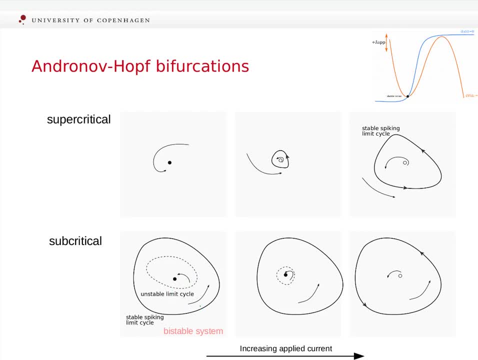 And then there is a stable limit cycle around it. So this system again is a bistable, or it is a kind of a neuron that at the same set of parameters can be either resting or spiking at a constant rate. 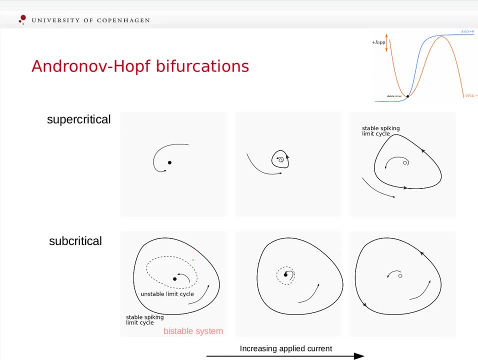 So it just depends on where we start from. If we start from within this unstable limit cycle, we will converge to a resting state, But if we start from outside of the unstable limit cycle- for example from here or actually from a more hyperparalyzed state- 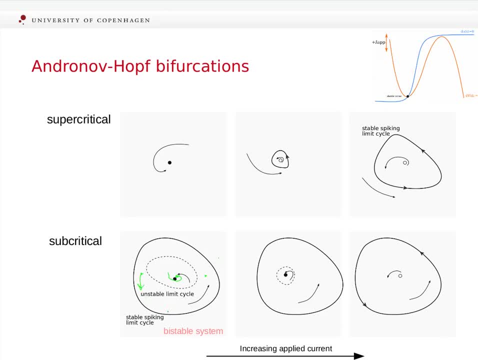 it will lead us to stable spiking. But as we increase the applied current, the unstable limit cycle becomes smaller and smaller and finally it shrinks right to the stable focus. and as it touches the stable focus it loses stability. So finally, just after the bifurcation, 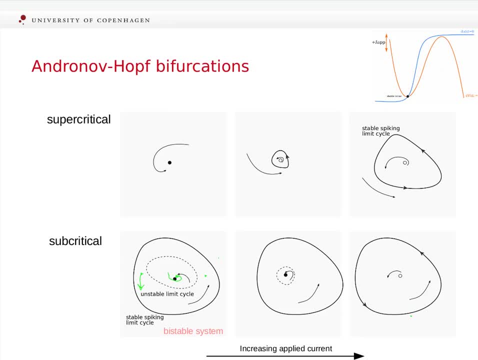 there is just an unstable focus and a stable limit cycle, And what we will see here is again a hard transition from resting to spiking, in contrast to a supercritical Andronov-Hopf bifurcation. So the case of the supercritical Andronov-Hopf bifurcation. 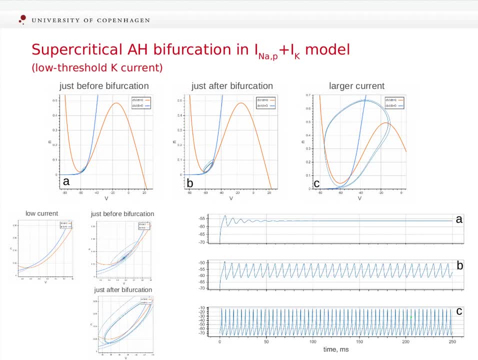 is illustrated in this slide. So again, this is just before bifurcation. Just after the bifurcation you see kind of subthreshold oscillations and at a larger current you have full amplitude action potentials And it's zoomed up in here. 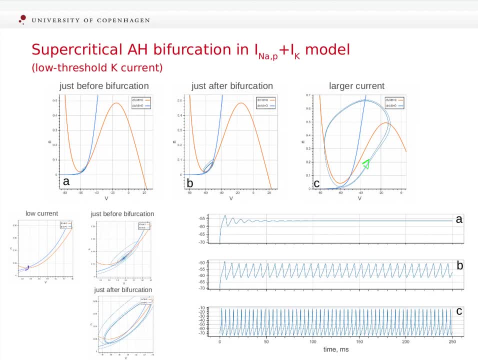 so we have, at low current or before bifurcation, stable focus and it's kind of converged to the stable focus point slower and slower. so the damping is actually less and less, and just at the bifurcation there is practically no damping. 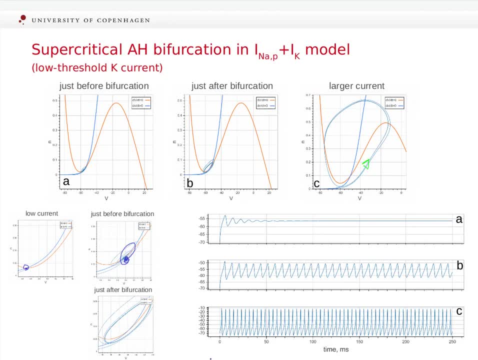 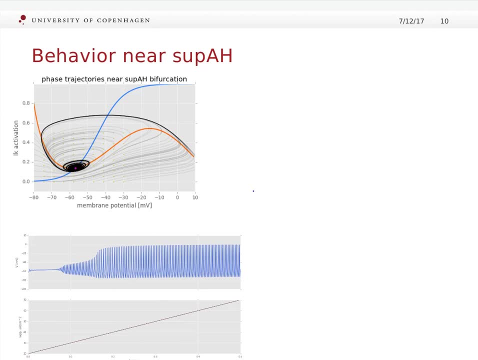 You have sustained subthreshold oscillations, but after the bifurcation at large current you have a high frequency spiking So near the supercritical Andronov-Hopf bifurcation. it doesn't matter where you start from. 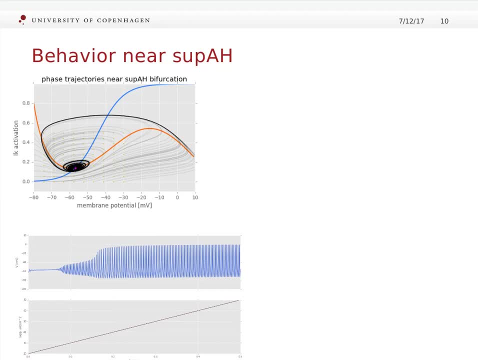 you will converge to a stable equilibrium or a stable resting state, but it depends where you start from. What depends on where you start from is whether you will have an action potential or just a subthreshold, oscillatory return to the resting state. So if you start, say, from somewhere here, 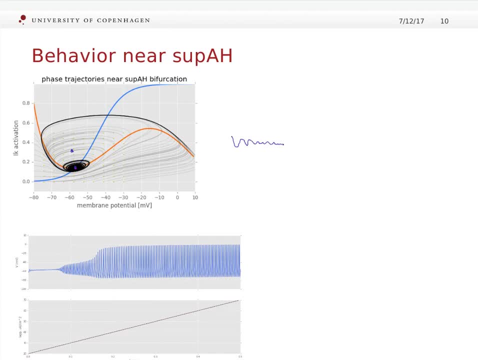 what you will observe is that you get decaying amplitude subthreshold oscillations in time. But if you start, for example- which is kind of counter-intuitively- if you start from a more hyperpolarized state, what you will get is an action potential. 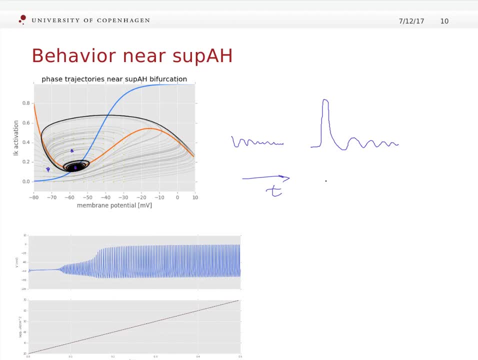 and then decaying subthreshold oscillations. So in here the concept of threshold for a neuron or spiking threshold is a more complex thing. It's, It's not that you depolarize a neuron and it can result in spiking. 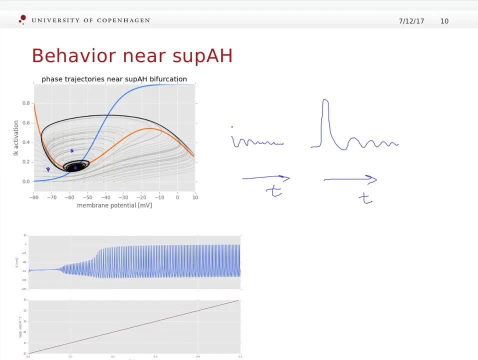 or an action potential. You can actually hyperpolarize a neuron and get an action potential. Now what happens if you start from a resting state and gradually increase the applied current, like shown in this figure? So this is our applied current. 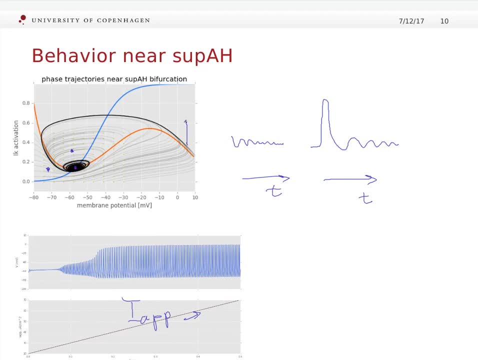 and it's getting more and more so. you shift your v-nuclein up and up. What you will observe is that first you are at the resting state, but then you get subthreshold oscillations with larger and larger amplitude, but relatively little, if any. 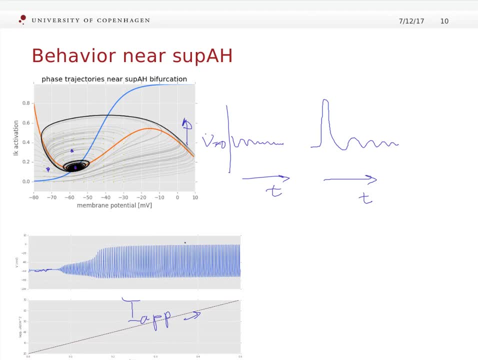 change in spiking frequency, but then you get full frequency sparks. So let me illustrate this in two videos. At first, we will look at the video with phase trajectories at different starting points And let me open this. So this is the video. 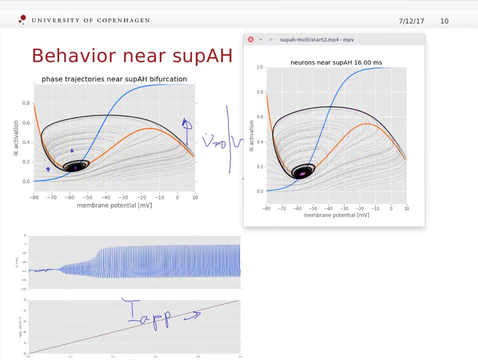 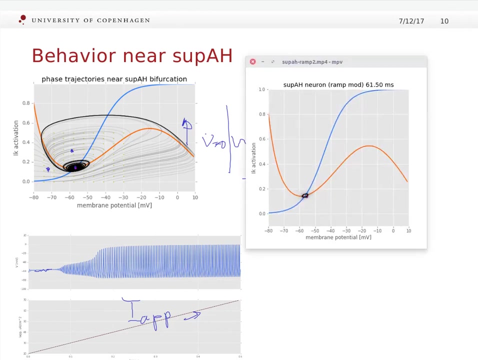 We start from a lot of different points and all trajectories end up in a resting state, But some of them do actually produce an action potential and some of them don't- Now what happens at the ramp stimulus protocol. So we start from a resting, stable focus. 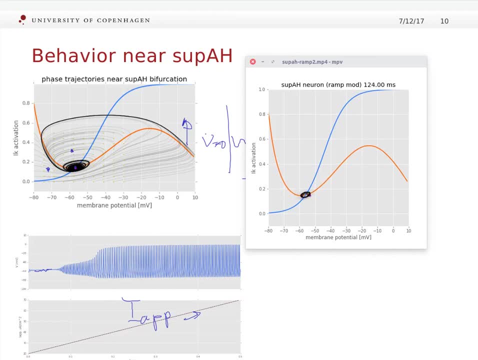 Here is our stable focus, but as we gradually increase the current, we get subthreshold oscillations with larger and larger amplitude but relatively same frequency, And finally we will get full-fledged spikes And you can observe that the rate of the increase. 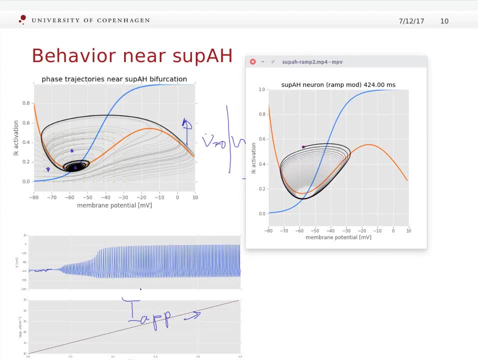 in applied current is different in this plot and in this demonstration. So here we go. We have real action potentials, But of course this concept of whether we have a real all-or-nothing response or not is blurred. So what is a subthreshold response? 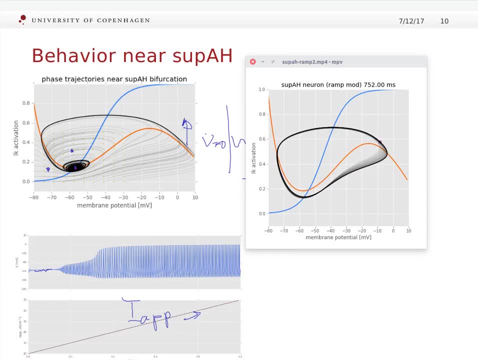 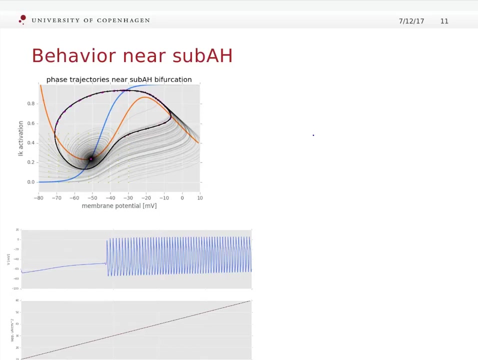 and what is a spike here is not a clearly defined thing. Right Next let's see what happens near subthreshold andronophobic bifurcation, And again, this system is bistable. So depending on where you start from, 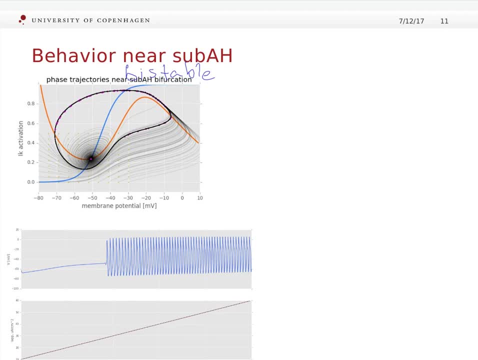 So you can start from somewhere here and result in a resting state with dynamics looking something like this: Or you can start from here and find a neuron producing spike Spikes at a constant rate at the same set of parameters. Let me show you this in a video. 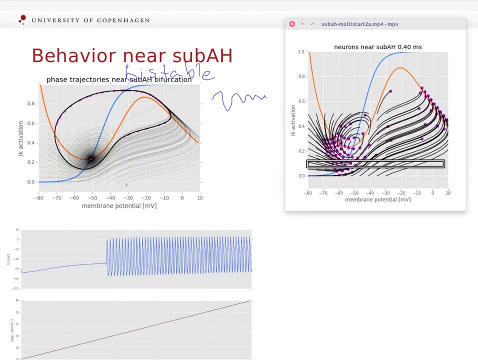 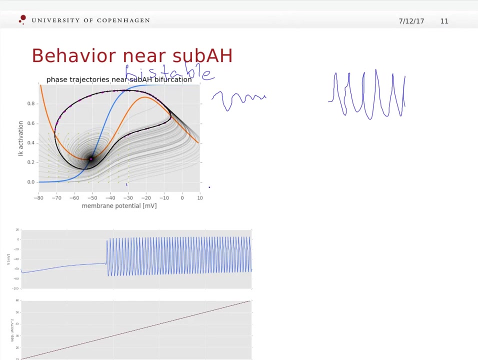 So here we go again. We start from a lot of different starting points and some of these starting points converge to a resting state and some stay on a sustained spiking regime. Now, what happens if we increase our applied current Right, Applied current getting larger and larger? 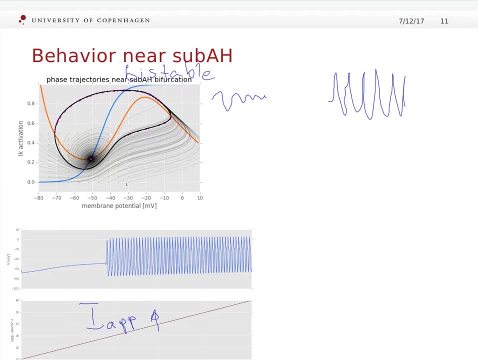 And I can show it in a video too. So basically, this is what happens. At first we are at a resting state. Gradually it gets Whoops And we have sustained spiking. Right Now what we have done here so far. 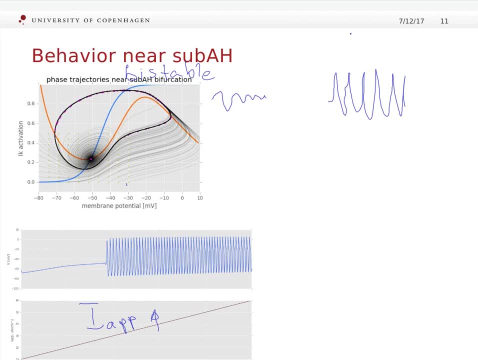 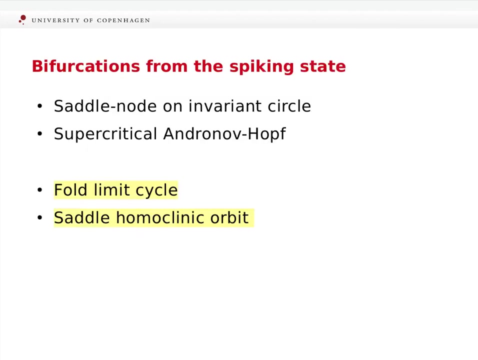 is. we analyzed the four scenarios of how a neuron can go from resting state to spiking state, So how a neuron can lose its stability. Now let's look at what happens as we go from a spiking state, or where do those limit cycles? 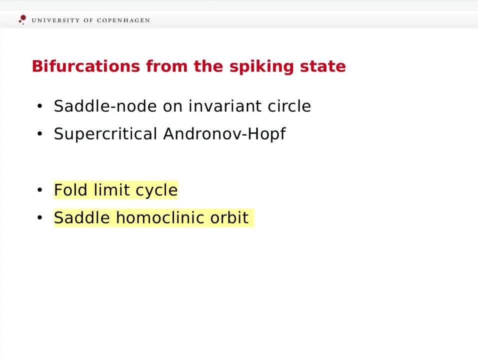 or stable spiking attractors come from. Again, there are four variants. The two of them are actually very simple. It's just the same as going from resting to spiking, but in a reverse direction. These are a saddle node, an invariant circle. 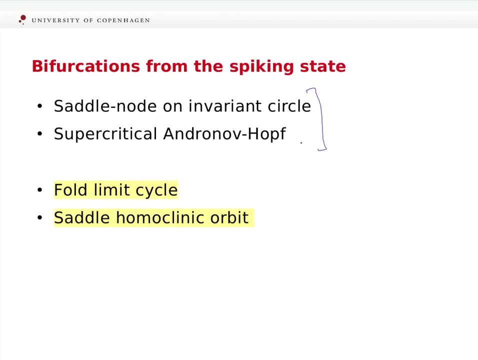 and supercritical andronoplast. These are supercritical andronoplast andronop-hop modifications. So if you go one way, like depolarizing the neuron or increasing or applying the depolarizing current, you get from resting to spiking. 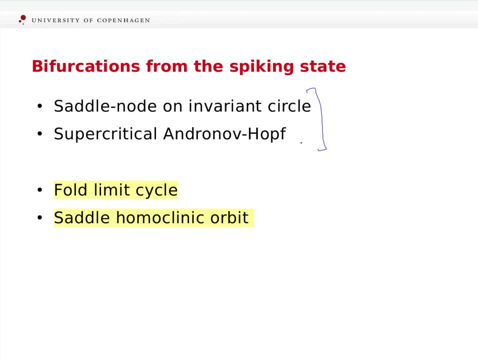 And if you inject a hyperpolarizing current, you go from spiking to resting in exactly the same manner. Now two other modifications are different. These are called fold limit cycle and a saddle node, saddle homoclinic orbit modification. Let's look at them in more detail. 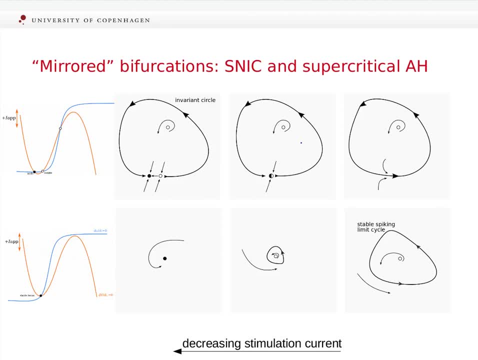 But first let's get through the mirrored modifications, The saddle node on invariant circle and supercritical andronoplast. So in this direction we are decreasing the stimulation current or injecting the hyperpolarizing current. Hyperpolarizing current, for example. 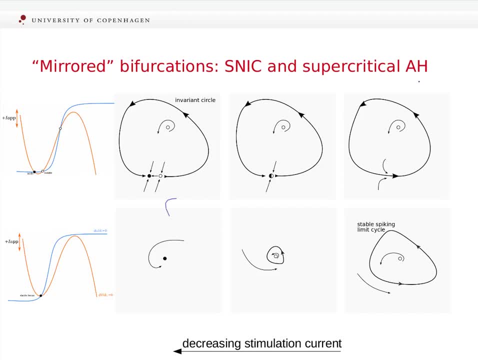 Again, we start from a spiking regime, but then our V-nuclein finally touches our N-nuclein. So just for. So this is our N-nuclein and this is our V-nuclein. So as the two nuclines touch, 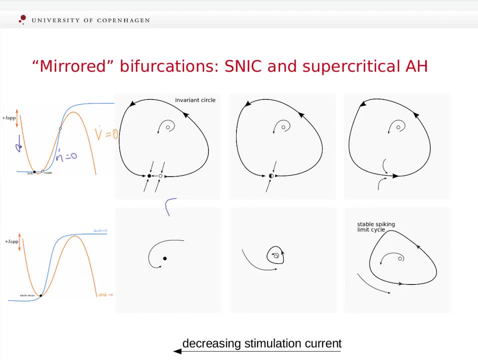 here, as we shift the applied current down, as we shift the V-nuclein down, we get the saddle, node, equilibrium point, and then the two equilibrium points are separated. So one is node and the other one is saddle. What we observe in dynamics: 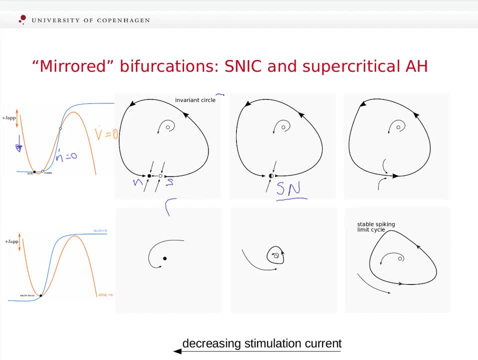 is a gradual decrease in the spiking rate. So at first we were spiking at the high rate, but then we get larger and larger interspike intervals because we get closer and closer in the narrow valley between the two nuclines And finally we get this saddle node. 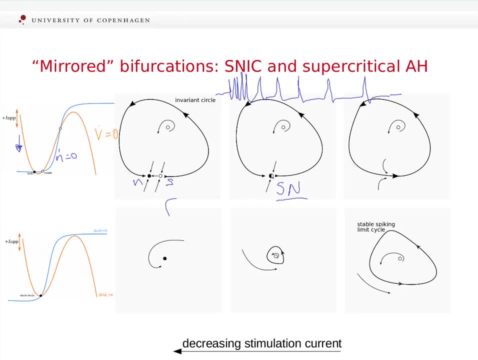 which is kind of an infinitely low frequency spiking, And then we just dwell in the resting state. Now, in the supercritical Andronov bifurcation from the spiking, we have a stable spiking limit cycle which gets smaller and smaller in amplitude. 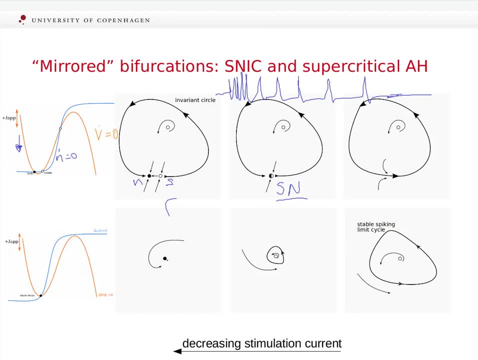 until it collapses onto the unstable focus. and the focus is now stable. What it means in dynamics is that at first we have full amplitude spiking, but then it gets smaller and smaller in amplitude and finally we have a resting state. Let's see it in actual simulation. 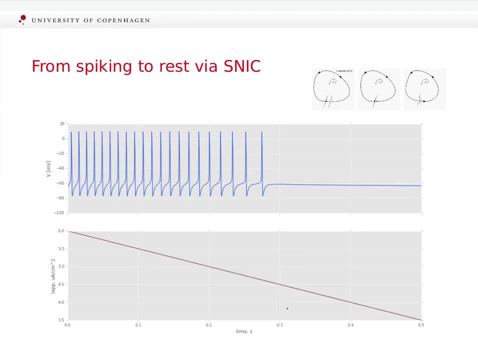 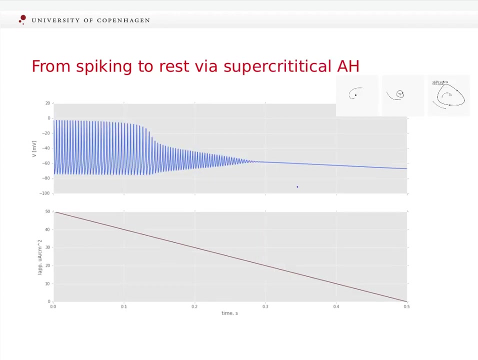 So we're going from spiking to resting state via saddle node and invariant circle. As we decrease the applied current we get larger and larger interspike intervals and finally the neuron stops firing. If we are going from spiking to resting state via supercritical Andronov hop bifurcation, 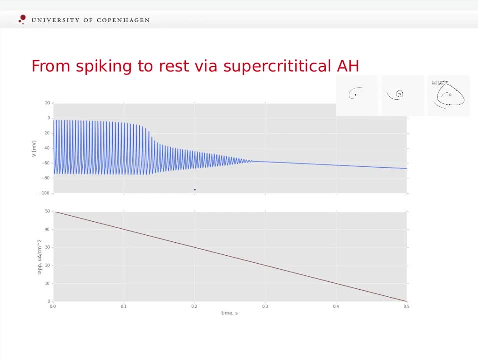 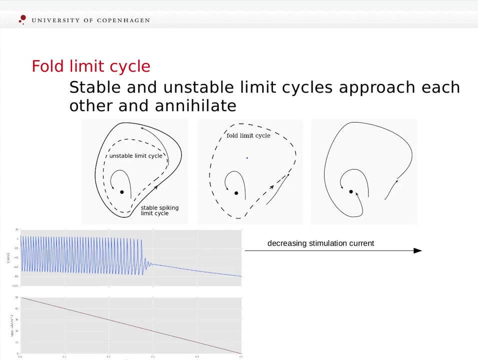 what we observe is little, if any, change in frequency, So the rate of spiking is kind of constant. here Again, here is an applied current and it goes down, But the amplitude of spikes gets smaller. Now in this system, 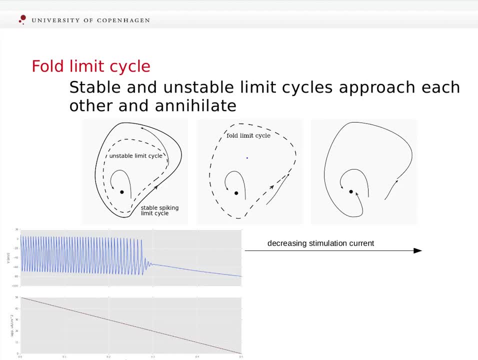 if we went from resting to spiking via supercritical Andronov hop bifurcation. we were talking about the coexistence of a stable limit cycle and unstable limit cycle and a stable focus. So if we have our decreasing stimulation current here, 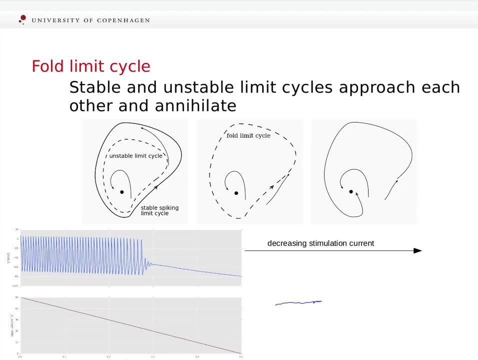 if we went from a resting state, so this was our stable focus- and then at the bifurcation point- so here the axis is actually the applied current- then it loses stability and unstable focus. I'll depict here with a dashed line, But at the same time: 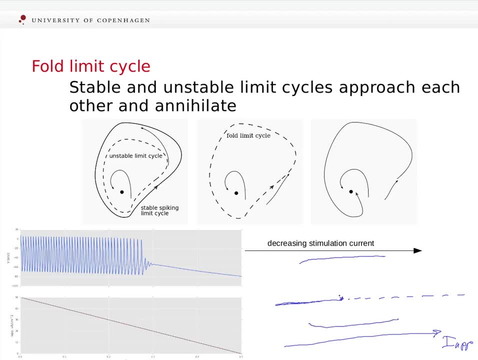 the system had stable limits cycle And here what I'm actually depicting is the range of the observed behavior. So you could think of it as the dynamics is jumping or going like this in time if we look at this in dynamics. So this would be: 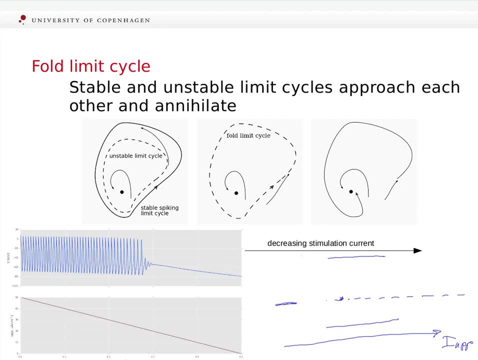 stable spiking. Oops, I didn't mean to delete this one. And here is the unstable limit cycle. Now, in the fold limit cycle, we are doing the same, but in the reverse. We are doing the same, but in the reverse. 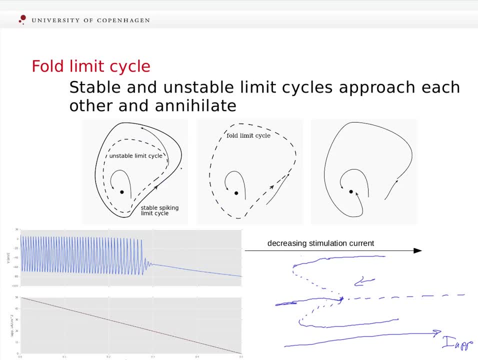 and what happens is the unstable cycle gets larger and larger in amplitude. So, like here, it gets larger and larger in amplitude. And then the two limit cycles merge, The unstable and the stable one, And as the unstable limit cycle touches the stable limit cycle, 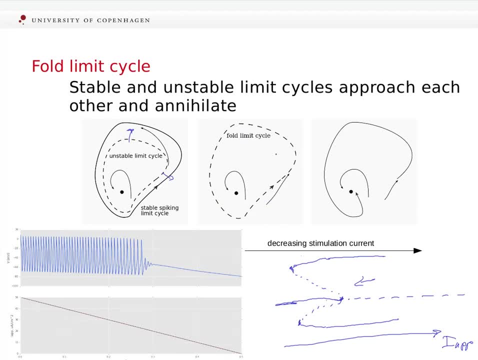 they both annihilate each other, And hence the name, the fold limit cycle, because it's kind of analogous to the fold bifurcation when a stable and unstable attractors or equilibrium points merge together. How it looks like in dynamics is that as we decrease, 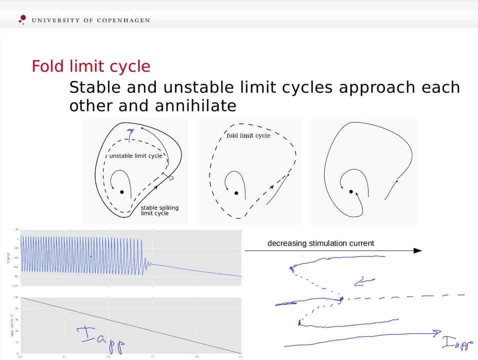 the applied current, we flip from spiking to non-spiking regime quite abruptly. So this is a hard transition from spiking to resting And I should say that there is little change in spiking frequency. Now, if we were losing stability. 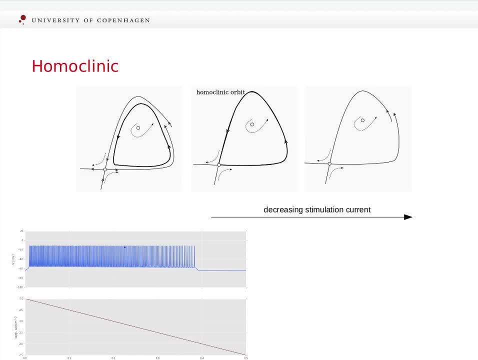 via the saddle node of invariant circle bifurcation. we had a coexisting spiking and resting state, So somewhere here was a stable node And we had a limit cycle attractor here. But as we decrease the stimulation, current the stable attractor. 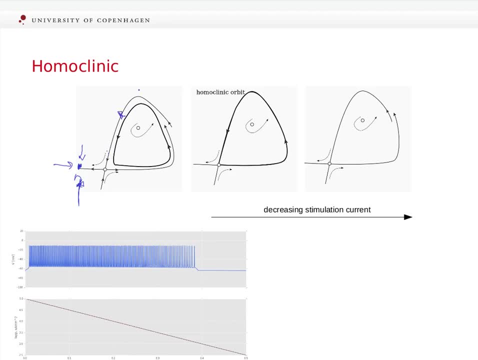 or a stable limit cycle, gets closer and closer to the stable manifold of the saddle And to the unstable manifold of the saddle, until it finally is merged in one corner with the saddle. And this is a homoclinic orbit because it starts and ends. 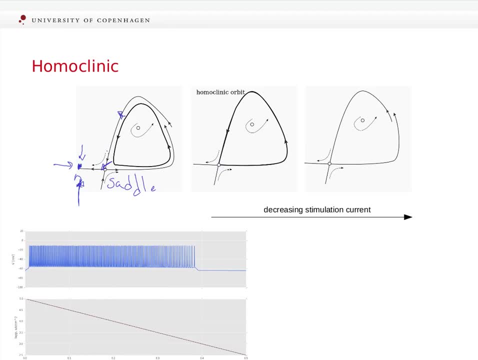 in the same point on the saddle. And finally, as we decrease the stimulation current even more, this homoclinic orbit starts and ends in the same point on the saddle And this limit cycle is unlinked. And now all trajectories, it doesn't matter.